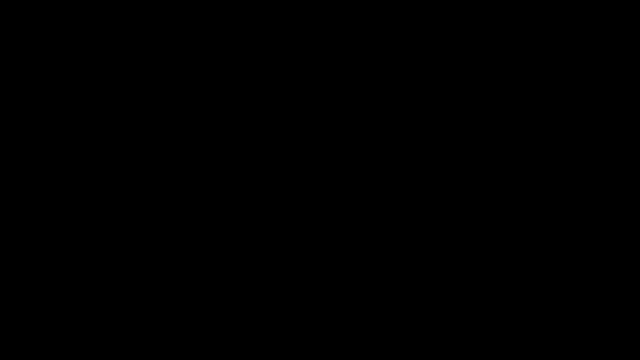 Yeah, as a teaching fellow, I've been helping with organizing and developing new content, mostly on the exercise side of the site, And the reason why we're doing this right now is you had some very interesting ideas or questions. Yeah, so as an Algebra teacher, 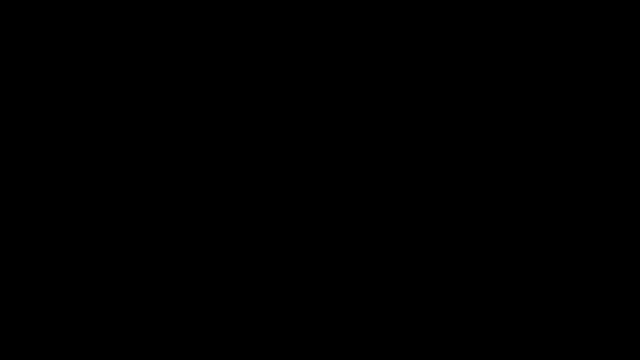 when I introduced that concept of Algebra to students. I get a lot of questions. One of those questions is: what's the difference between an equation and a function, The difference between an equation versus a function? It's an interesting question. Let's pause it and see. 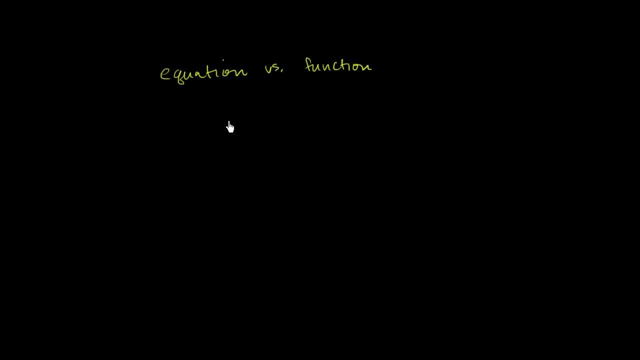 Let the viewers try to think about it a little bit, and then maybe we'll give a stab at it. Sounds great. So, Sal, how would you answer this question? What's the difference between an equation and a function? Let me think about it a little bit. 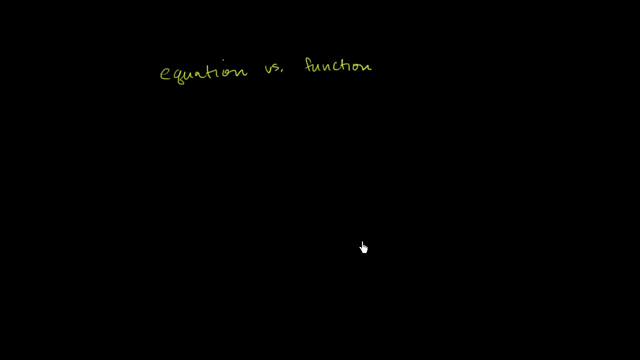 So let me think. I think there's probably equations that are not functions and functions that are not equations, and there are probably things that are both. So let me think of it that way. So let's first think of it. So I'm going to draw, if this is the world of equations. 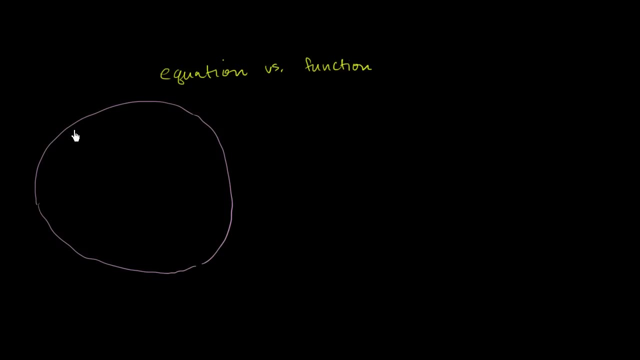 right over here. This is the world of equations. so this is equations, and then over here is the world of functions. That's the world of functions. I do think there is some overlap. We'll think it through where the overlap is. 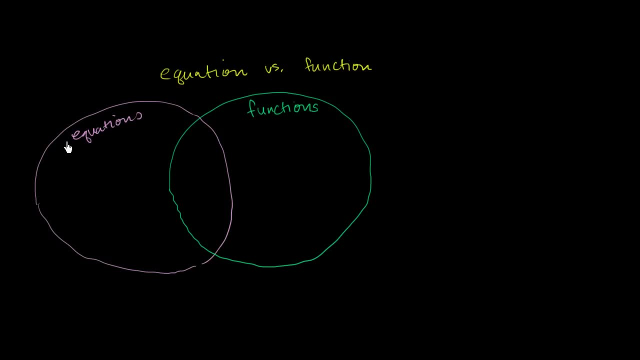 The world of functions. So an equation that is not a function that's sitting out here, I think a simple one would be something like: x plus 3 is equal to 10.. I'm not explicitly kind of talking about inputs and outputs or relationship between variables. 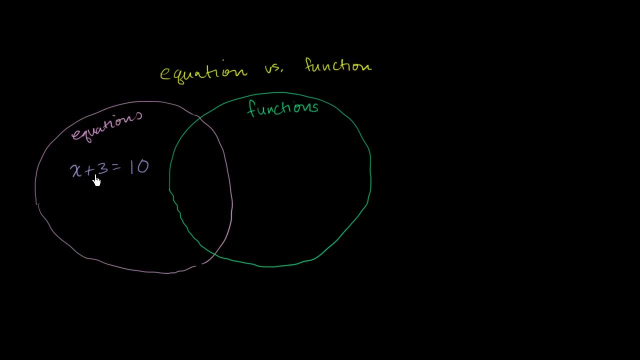 I'm just stating an equivalence. the expression x plus 3 is equal to 10.. So this, I think traditionally would just be an equation, would not be a function. Functions essentially talk about relationships between variables. You get one or more input variables. 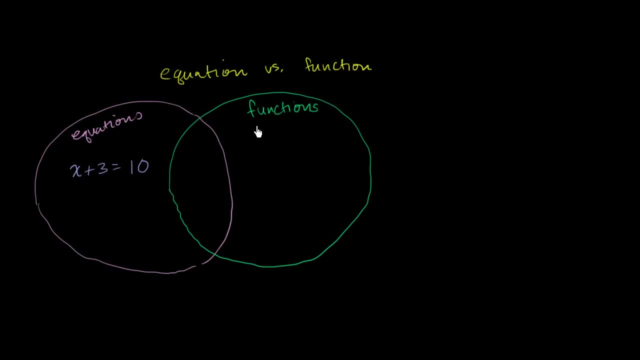 and it will give you only one output, variable output value. And so you could have something like: and you can define a function, and I'll do that in a second- You could define a function as an equation, but you can define a function a whole bunch of ways. 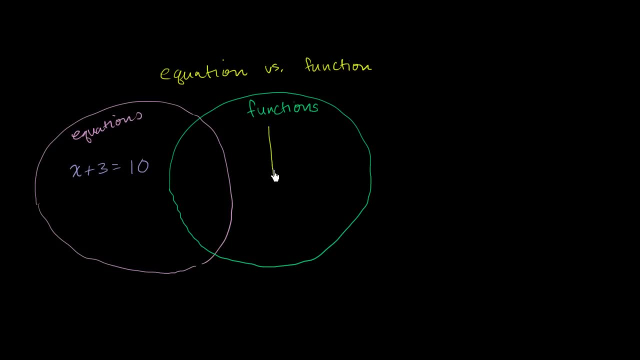 You can visually define a function, maybe as a graph, So something like this, where maybe I actually mark off the values. So that's 1,, 2,, 3.. Those are the potential x values And then on the vertical axis I show.